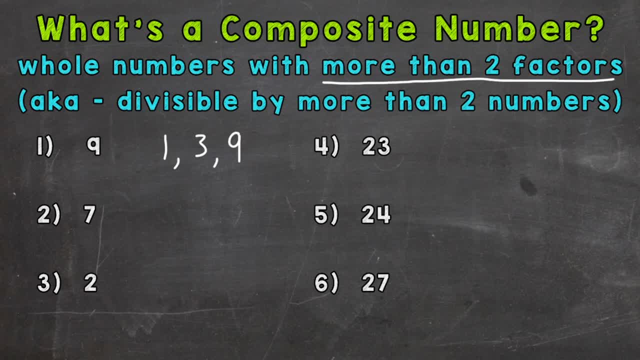 more than two factors, Or it's divisible by more than two numbers- Nine is divisible by one, three and nine- Or think of it as one, three and nine go into nine, So nine is composite. So let's move on to number two, where we have seven And we need to think of the factors of. 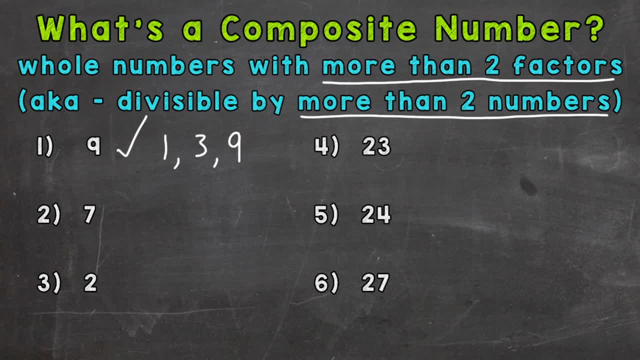 seven. So what numbers go into seven, Or what numbers multiply together to equal seven? Well, we know, one times seven equals seven, And that's actually the only two factors that go into seven. So what numbers go into seven? Well, we know, one times seven equals. seven. So what numbers go into seven? Well, we know, one times seven equals seven. And that's actually the only two factors that go into seven. So what numbers go into seven? Well, we know, one times seven equals seven. So what numbers go into seven? Well, we know, one times seven equals. 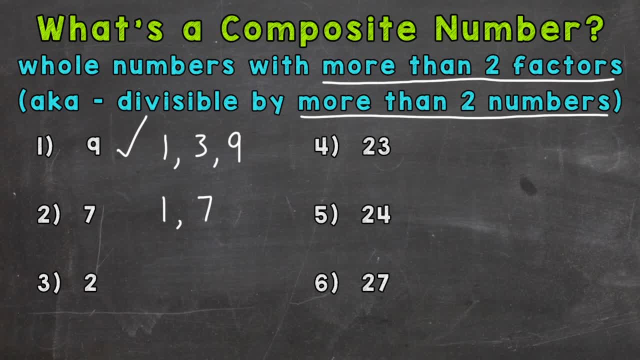 of seven. Seven only has two factors, so it's not composite. If a number only has two factors, it's called a prime number. Now I have a video going into further depth on prime numbers. I'll drop that link down in the description. On to number three, where we have two. Now, two is a. 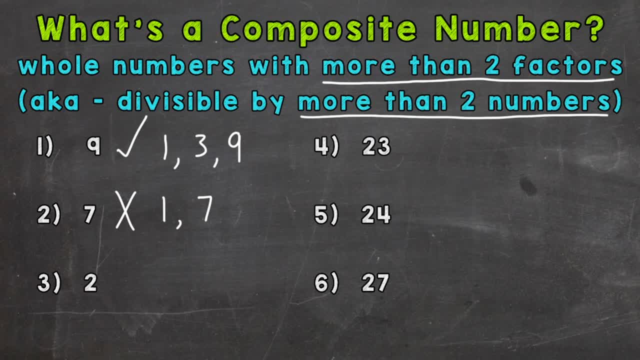 unique number here And we'll find out why in a second. So the factors of two: well, one times two equals two And there aren't any other factors of two. So one and two are factors of seven And are the factors of 2.. 2 only has two factors, so 2 is prime, just like 7, but 2 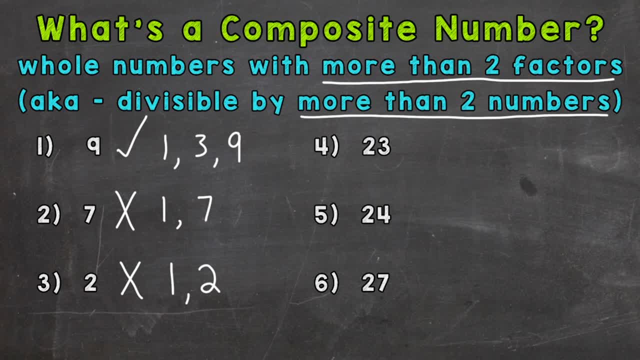 is unique because it's the only even number that is prime. All other even numbers are automatically composite because we have the factors of 1 and the number itself, and then 2 is an automatic factor of all the other even numbers, On to number 4, where we have 23.. So 23, we need to think of its factors. What? 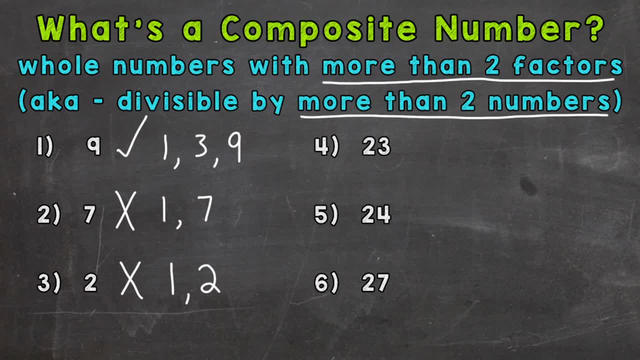 numbers can we use to equal 23?? Multiply together to equal 23.. Well, 23 only has two factors: 1 and 23.. So 23 is prime as well. It is not composite On to number 5, where we have 24.. Now we can tell that 24 is composite right away because it's an. 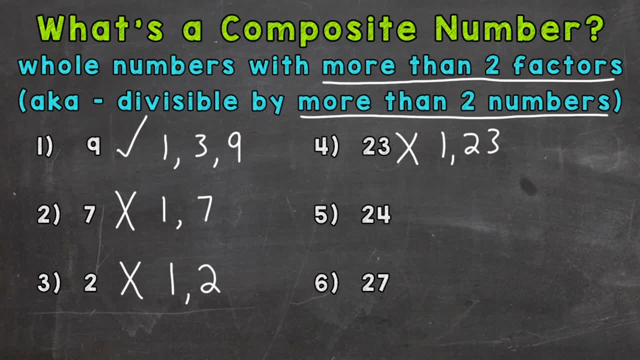 even number. We know that 1 is a factor, 24 is a factor and then 2 is a factor. So right off the bat we know that 24 has more than two factors, therefore composite. But we will list them out just to see how many different factors 24 has. So we know.